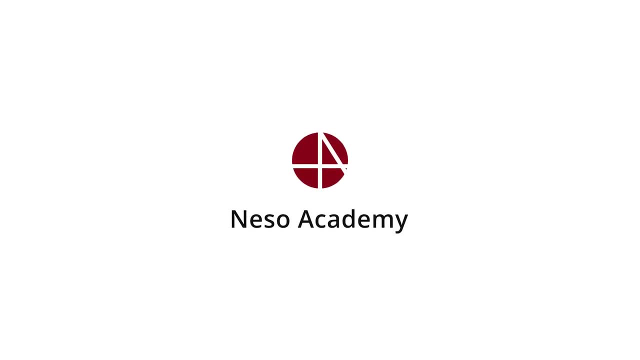 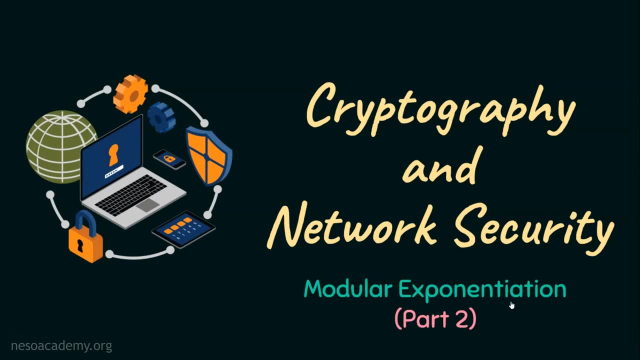 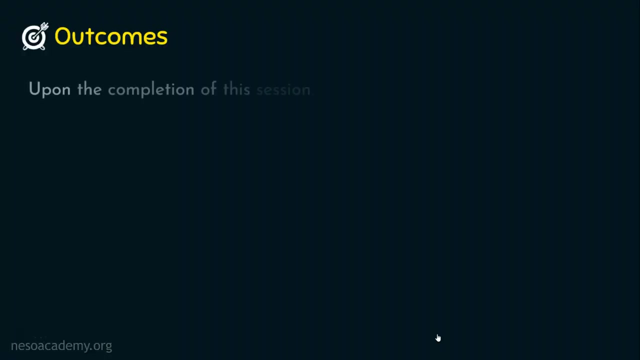 In the last presentation we have seen part one of modular exponentiation. In this presentation we will focus on the part two of modular exponentiation. So in this lecture we are going to exclusively focus on understanding modular exponentiation with examples, That's. 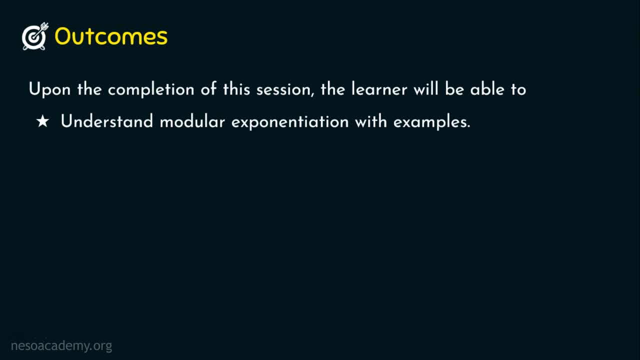 the only outcome of today's lecture. Before we dive into solving the problems of modular exponentiation, I want to state this firmly: Modular exponentiation is really an important topic to be addressed and to be learned meticulously In order to solve problems pertaining to the most popular and widely used cryptographic algorithms, such as the. 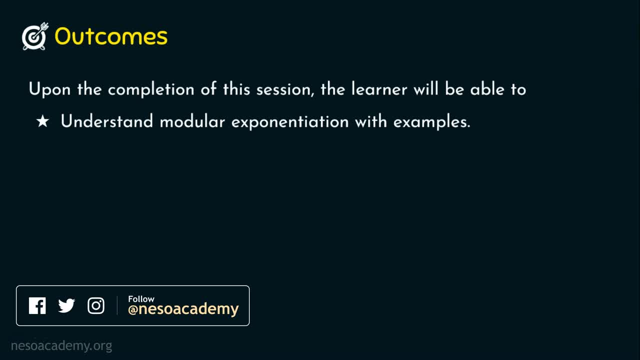 Rivest-Shamir-Adelman algorithm, Simply RSA algorithm, the Diffie-Hellman Key Exchange algorithm, the Elliptic Curve cryptography, the Rabin cryptosystem and other algorithms as well. we need the following: We need the strong foundations of modular exponentiation, So I request everyone to 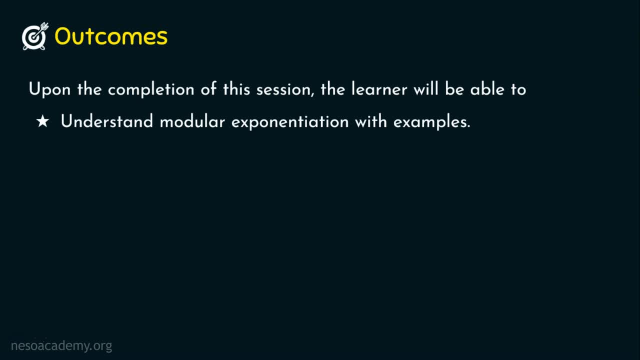 work it out parallelly with me so that you will gain better insights about solving the problems of modular exponentiation. Why waiting? Let's dive into example number one. The question is: Solve 88 power 7 mod 187.. See, if you observe, in the last presentation we have seen this. 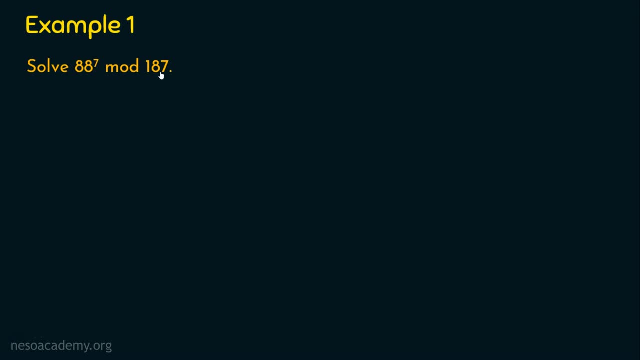 number and this number are close to each other and that's why we were able to solve those questions so quickly. The difference between this number and this number was not a big difference in the last presentations, But we can't expect questions to be easy always. 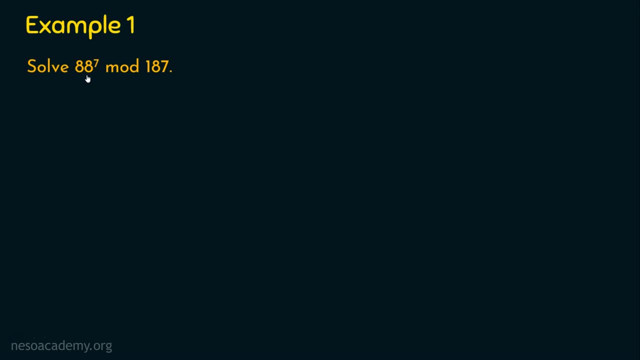 Sometimes we may get questions like this also, where the difference is very big. Can you see here, This is 88 and this is 187.. So we want to know how to solve these kind of big differences also. So let's understand how to solve these kind of problems as well. 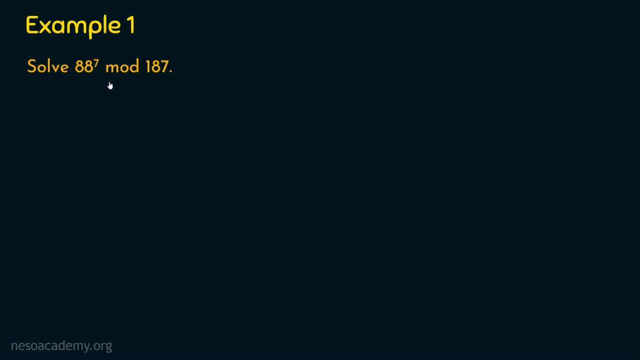 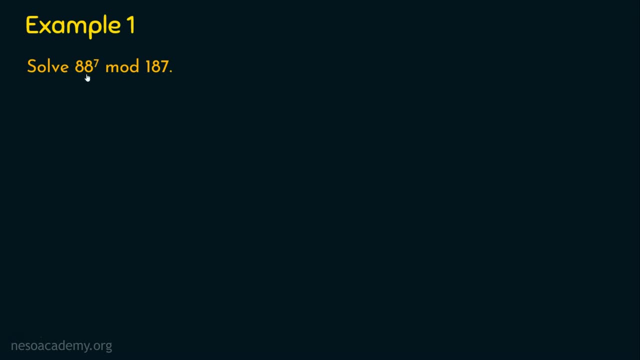 example number one. now I will tell you this: short power. So always we are going to start with the base power 1.. Then we will be doubling it. For example, if this is 88 power 7, then we are going to start with 88 power 1.. Then we will get the 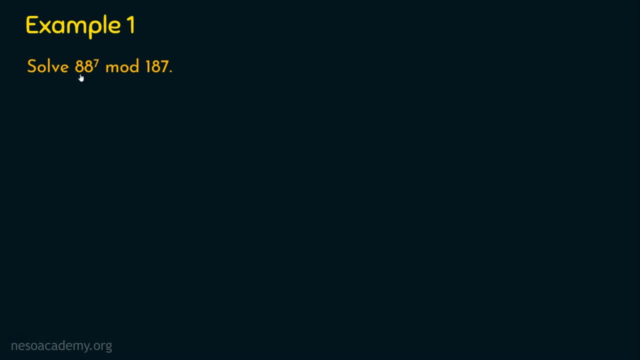 result for that. Then we will do 88 power 2, 88 power 4,, 88 power 8,, 88 power 16,, 88 power 32,, 88 power 64,, 88 power 128, and it goes on. Obviously we are not going to do this infinitely. 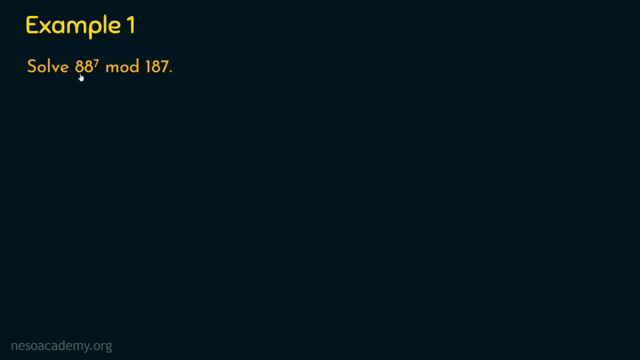 right At some point of time. we are going to stop When we are going to stop that. We will be stopping this process till we get this number right. Now you may be asking me a question: We are going to double it. Will we be exactly getting this number? No, So we are going to. 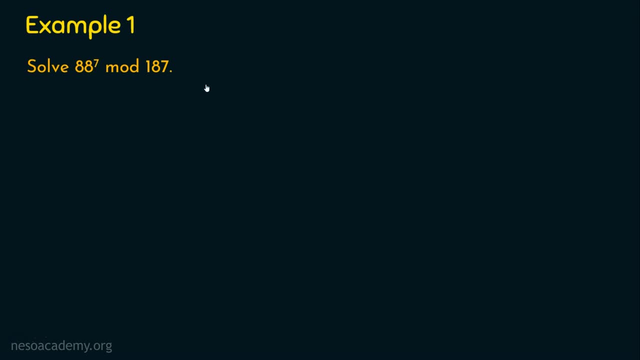 stop the process before we get this number. I will explain this. No worries, Let's solve this problem now. So obviously we are going to start with 88 power 1, right? So see here. the question is 88 power 7 mod 187.. 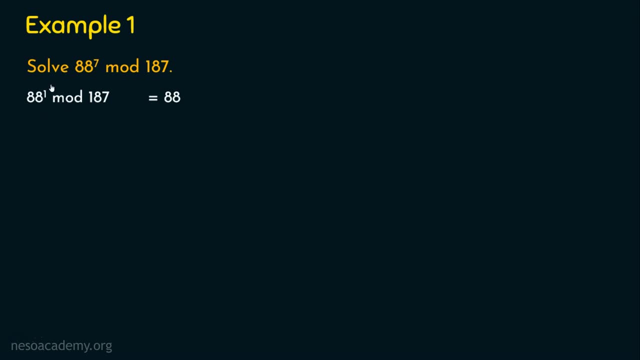 So let's start with 88 power 1 mod 187.. So 88 power 1 is 88.. So I am simply using 88, right, You can also use negative representations also, But here the negative number or the minus number. 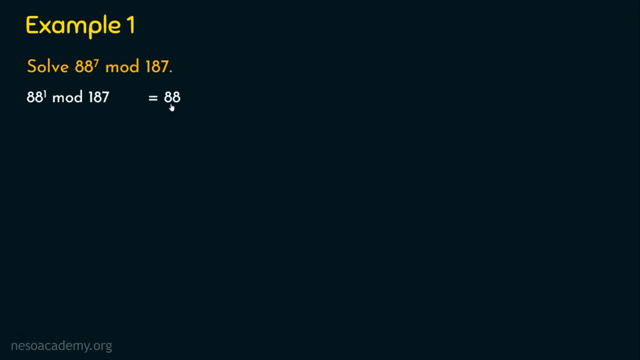 will be a bigger number. So I am just taking the positive number only. Anyway, in the coming examples I will also take some negative numbers and I will show you how easily we can solve these problems. In this case we are just taking 88. power 1 mod 187 is equal to 88.. Completed right. 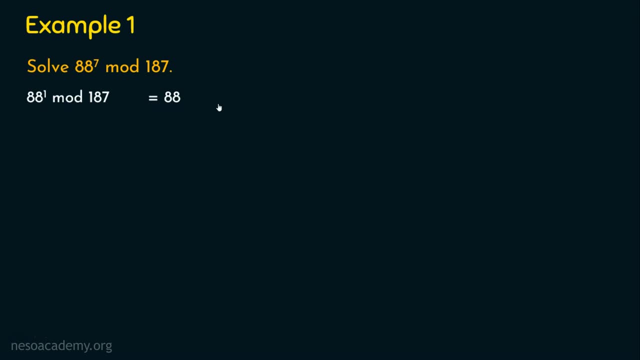 Hope this is clear. We started with 88 power 1.. Then we need to proceed with 88 power 2.. How can we write 88 power 2?? So we are doing 88 power 2 mod 187.. How can we write 88 power 2 with the? 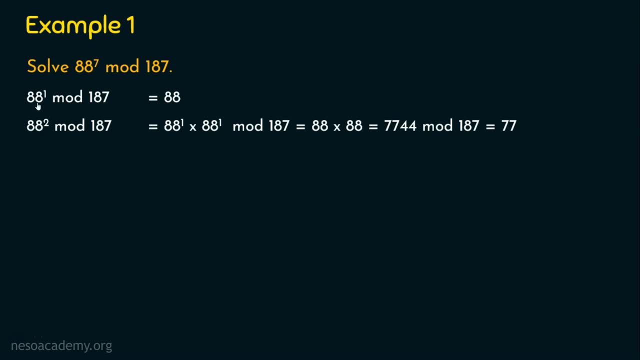 help of previous step. 88 power 2 can be written as 88 power 1 multiplied by 88 power 1, right, Because when the base is common, 88 is common and we can add the powers right. So 88 power 2 can. 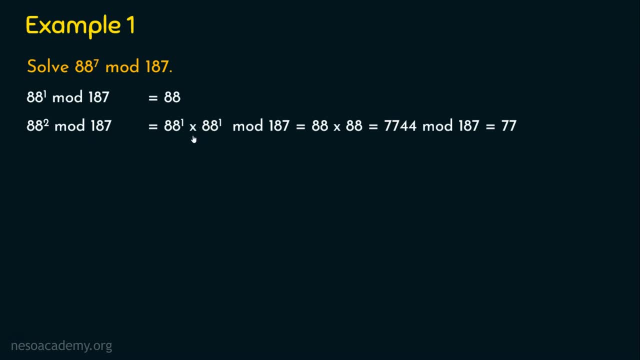 be written as 88 power 1 into 88 power 1 mod 187.. So this is equivalent to this, isn't it? So already in the previous step we got it. what is 88 power 1 mod 187, which is 88, right? So just replace this 88 power 1 as 88 multiplied by 88. 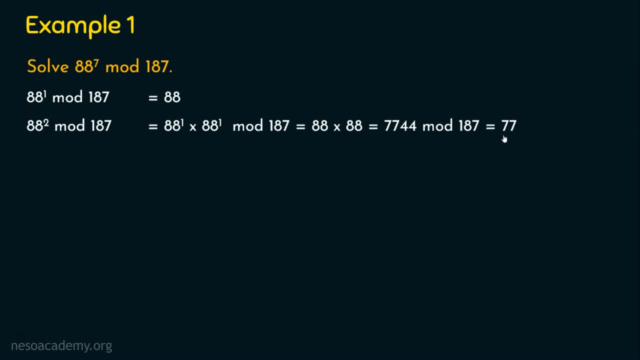 which gives double 7, double 4. Perform mod 187.. We will be getting the remainder as 77. So 77 is the answer for 88, power 2 mod 187. Then we are going to double this right. We just did it. 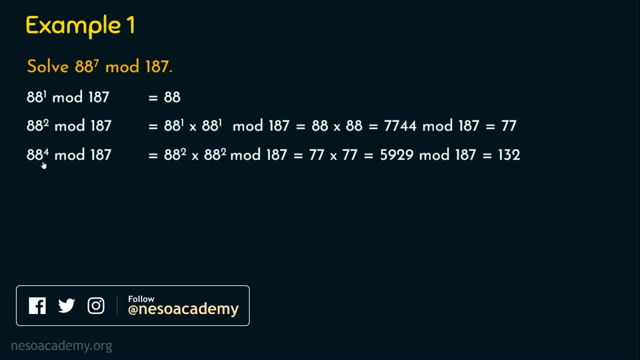 for 88 power 4, right, So I am just doubling this. So 88 power 4 mod 187 is equal to 88 power 2 multiplied by 88 power 2.. You can notice here this 88 power 2 will be the previous step, right This? 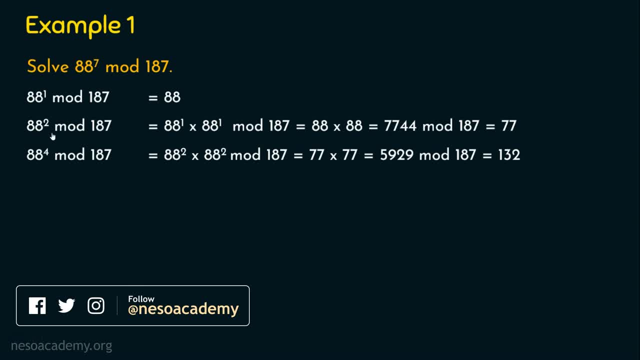 is 88 power 2.. What we have found for 88 square, That is this: We found it as 77, right? So I am just using 77 multiplied by 77, which gives 5929 mod 187.. When you simplify this, you will be. 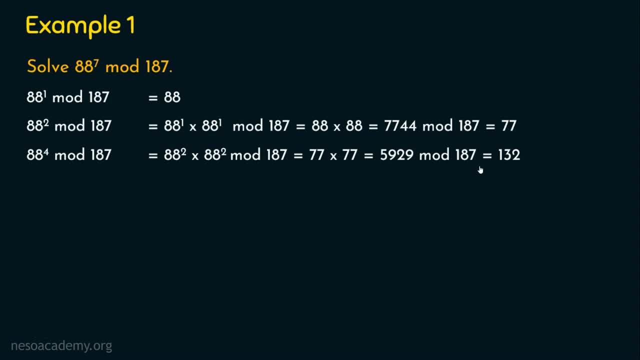 getting 132.. Then we need to double it right. So 88 power 8.. Remember, are we going to do 88 power 8? No, because our question is: it is 88 power 7.. So we are going to stop up to this. Now we can get this 88 power 7 with the. 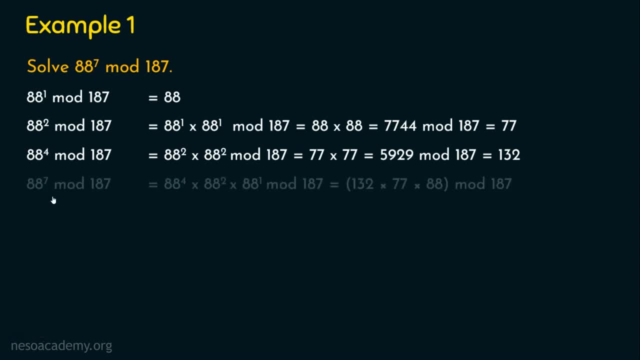 help of previous steps. Can you understand this? Just see, 88 power 7 can be written as 88 power 4.. That is this previous step, multiplied by 88 power 2, which is this, multiplied by 88 power 1, which is this, Since the base is common. 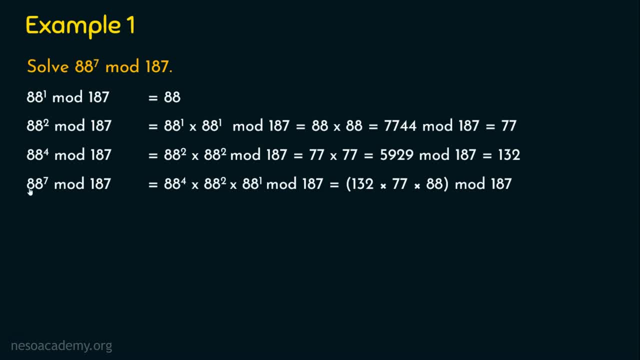 you can add the powers right: 4 plus 2 plus 1 is what 7.. So 88 power 7 can be rewritten as 88 power 4 multiplied by 88 square, multiplied by 88 power 1 mod 187.. So we know what is 88 power 4.. In the 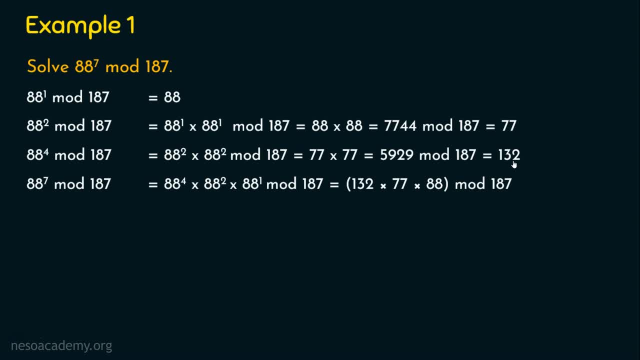 previous step we found it right: 88 power 4 is 132.. So 132 multiplied by what is 88 power 2? This step right. So here we have 77. So I am using 77 and the last one is 88 power 1.. What is? 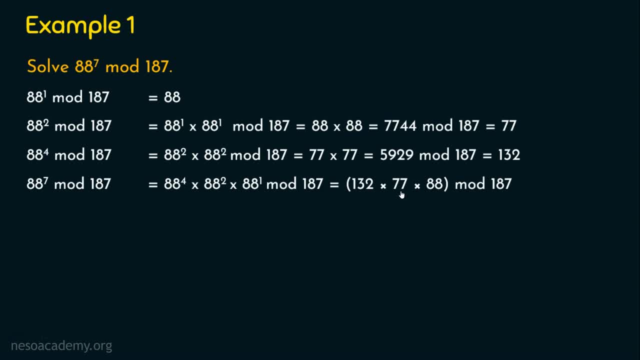 78?. So we get 132 multiplied by 77, multiplied by 88 mod 187.. Just simplify this. we will be getting this value Perform mod 187, the remainder will be 11.. So the answer for the question 88 power 7. 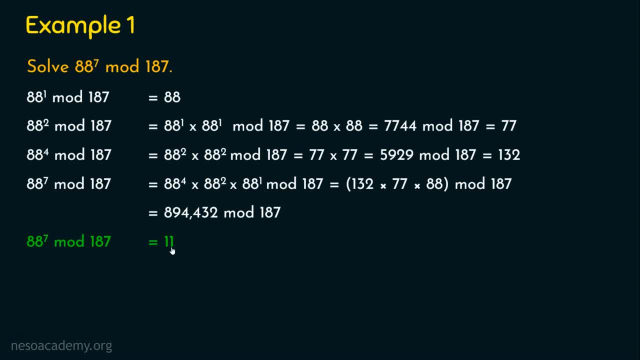 mod 187 is 11.. Before we step into example number 2, I want everyone to mark this example 1 because in the coming chapters I will be solving RSA problems. obviously, There I will be taking values from the RSA problems, which results in evaluating an expression 88, power, 7 mod 187, which is exactly. 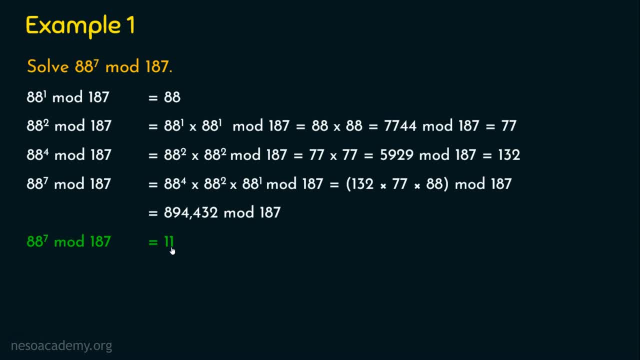 this question During the time of solving that particular RSA problem, I will definitely let you know to refer this particular example 1.. In turn, we can save some time there. I know it will be somewhat difficult to understand in example number 1 itself, So let's move on to example. 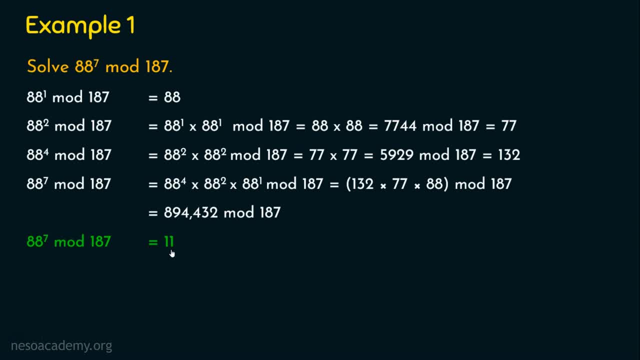 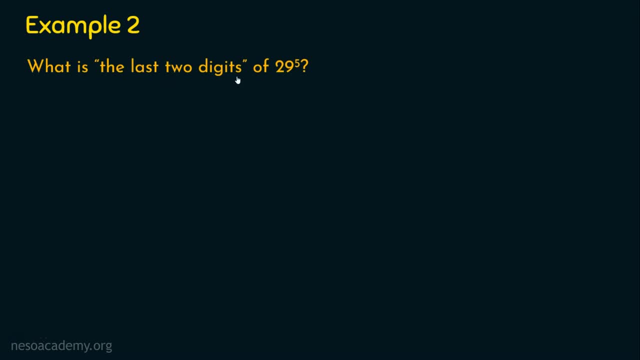 number 2 with a different question, but still, the logic is the same. Let's see that now. Example 2.. The question is: what is the last two digits of 29 power 5?? Oh, where is the mod I didn't give? 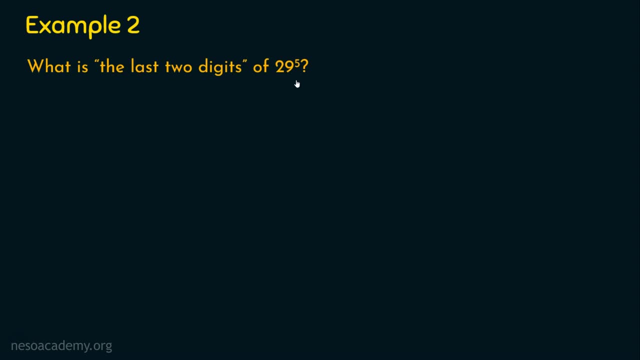 any mod value, right? So what we can do, Are we going to seek the calculator for doing this? If we are going to do it in a calculator, we can get the result and the last two digits. we can easily get it. But we are going to follow the modular exponentiation methodology. So we are going to 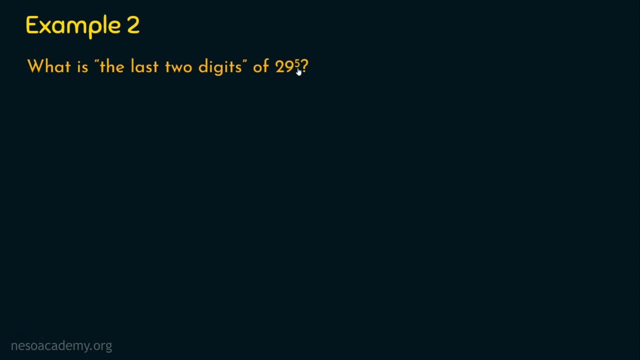 start with 29, power 1.. But what is the mod value? It's very simple. We are going to take the last two digits. Say, if you get a number, when you will get the last two digits? When you divide that number by 100, right? So whenever you divide any number by 100, the 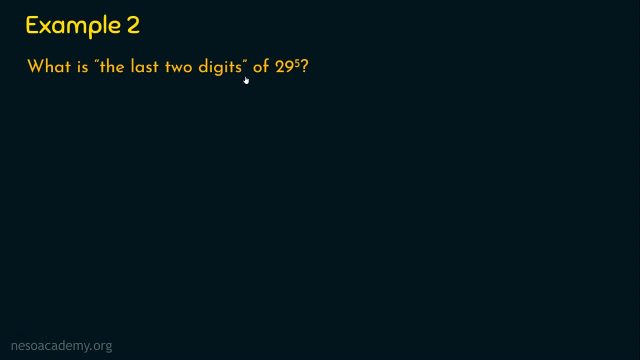 remainder will be definitely between 0 and 99.. That's for sure, right? So the question which is: what is the last two digits of 29 power 5 is equivalent to solve 29 power 5 mod 100.. In case. 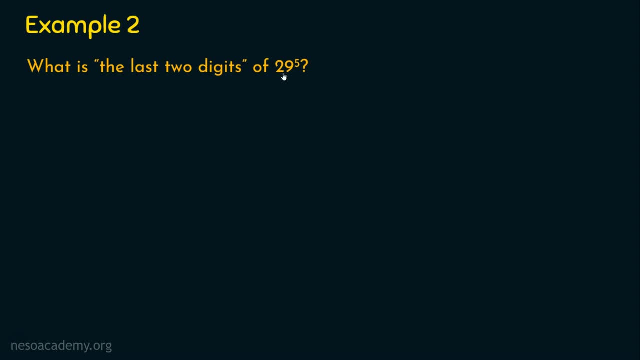 you get the last two digits of 29 power 5, you can modify this question as either 29 power 5 mod 100 or 29 power 5 mod 10.. Even you can do mod 1000 also. Just take the number of digits as mentioned. 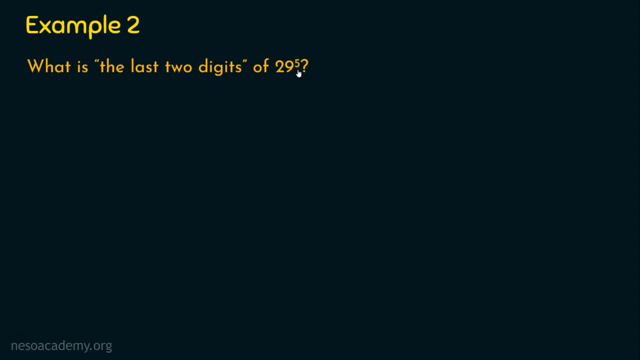 in the question. In this question also we can use 29 power 5 mod 1000.. We will be getting some result and obviously we are going to take the last two digits only. You can solve it like 29 simplification, right. We are going to take only smaller numbers for easy calculation and that's. 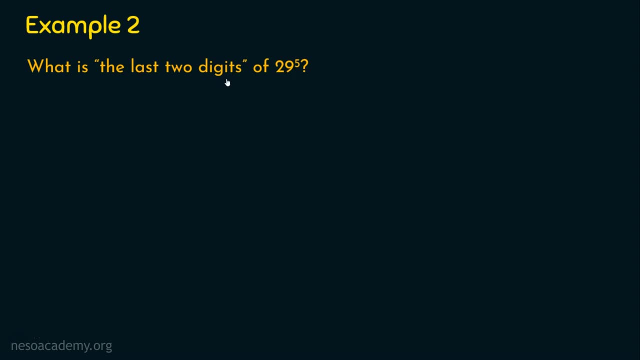 why I recommend you to solve these kind of questions with smaller numbers. So the question is actually: 29 power 5 mod 100, right? Okay, let's start it now. Obviously, we'll be starting with power 1, right? So we are going to start with 29 power 1.. So 29 power 1 mod 100, which is equal to: 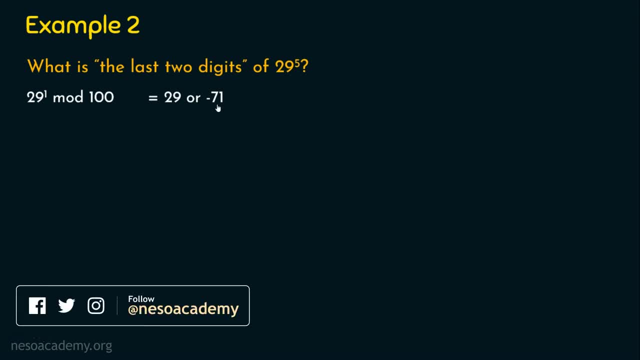 29 or we can also represent in the minus right. In the previous example I didn't solve it with minus. I told you that in the coming examples we'll be solving it. So just see 29, power 1 mod. 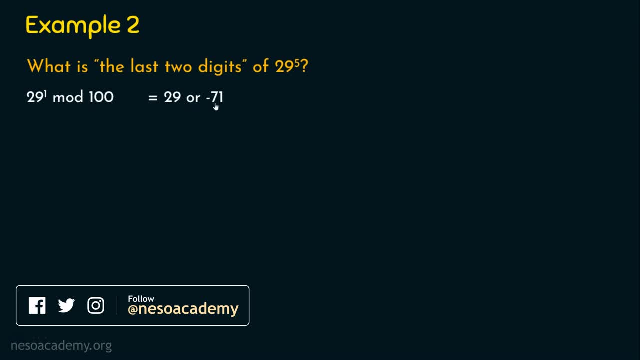 100 can be either 29 or minus 71, which is smaller In terms of value. minus 71 is smaller, but if you take minus 71, do you think minus 71 multiplied by minus 71 is easier when compared to 29 multiplied? 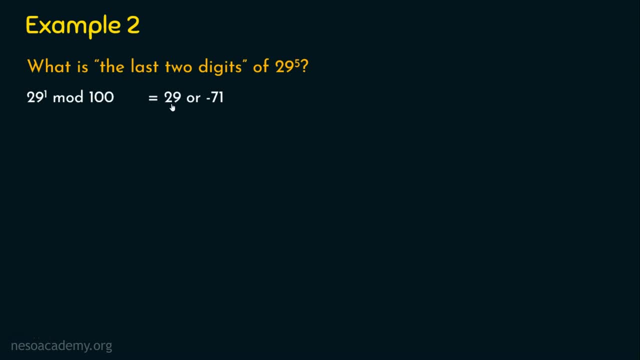 by 29?? We will take 29, which will be certainly easy for doing the calculations. So step number one is 29, power 1 mod 100 is 29.. So let's start with 29 power 1 mod 100.. So let's start with. 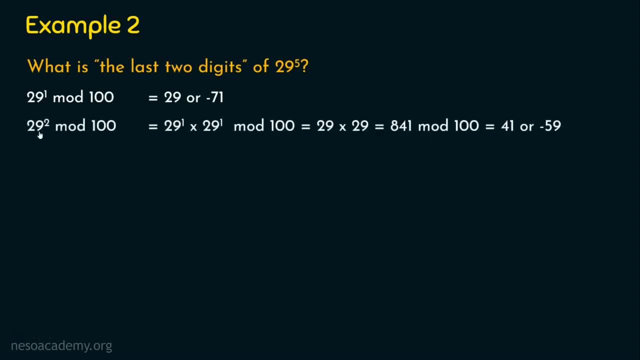 29 or minus 71.. So step number two is 29 power 2 mod 100, right, 29 power 2 can be written as 29 power 1 multiplied by 29 power 1 mod 100 remains the same We already calculated in the previous. 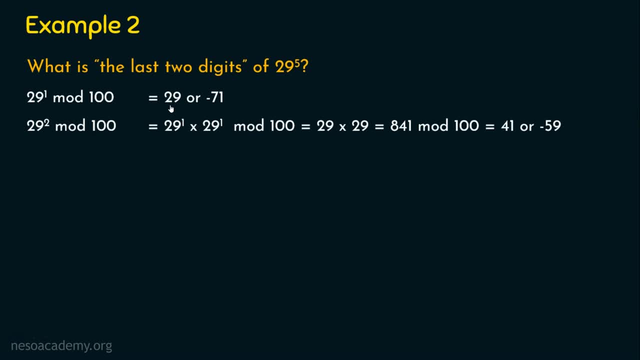 step We can take either 29 or minus 71. Since 29 is easy for doing calculations, I'm preferring 29.. So I'm using 29 multiplied by 29, which gives 841 mod 100.. So the result of this can be either 41. 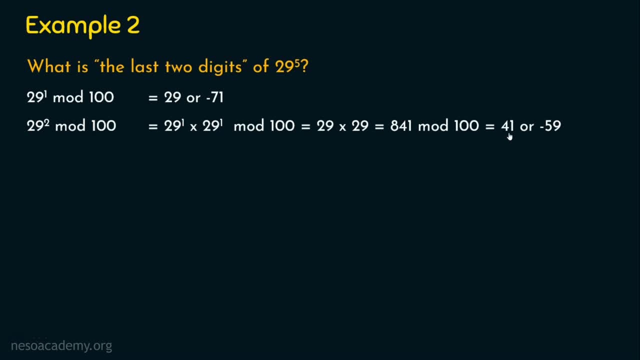 or minus 51. So let's just take 49.. So 841 when it is divided by 100, we get 41. So we can have minus 59 also, But anyway, we are going to take only 41,, not minus 59.. So let's move on to the. 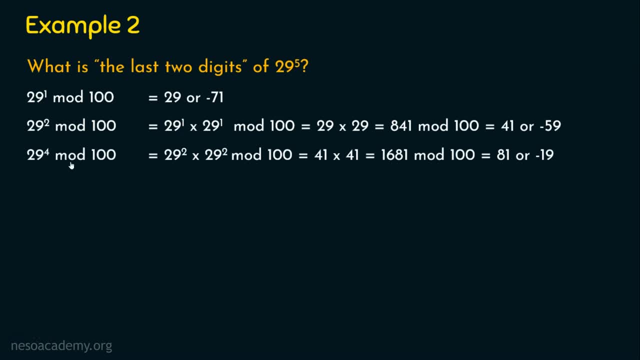 next step, which is 29 power 4.. So 29 power 4 mod 100 can be written as 29 square multiplied by 29 square mod 100.. We know 29 square is 41.. So 41 into 41, which is 1681 mod 100, which gives 81, or. 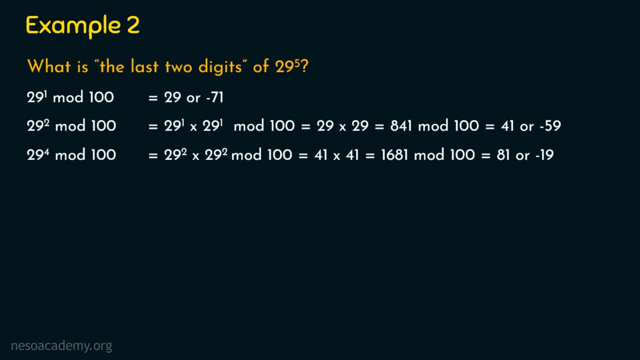 minus 19,. right, Then we are not going to calculate the value of 841.. So let's start with carrying out 29 power 8, because we are going to find only 29 power 5.. So we are going to stop. 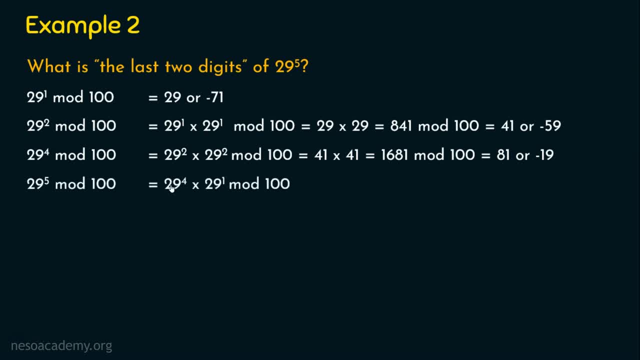 with this. So 29 power 5 mod 100 can be 29 power 4, which is this step, and we don't need this step now, We need only this right. So 29 power 4 multiplied by 29 power 1.. So 4 plus 1 is 5.. 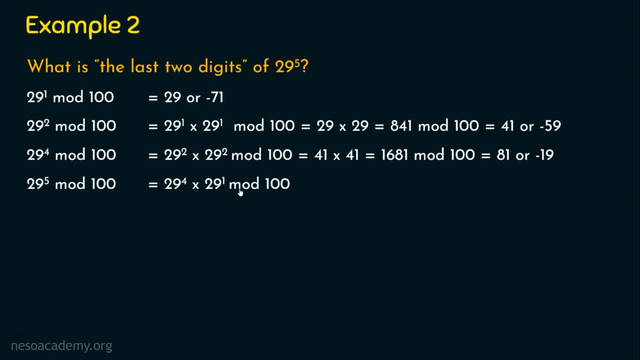 So this is perfect. So 29 power 4 multiplied by 29 power 1 mod 100.. We know what is 29 power 4.. It can be 81 or minus 19,. right, Because 29 power 4 is. 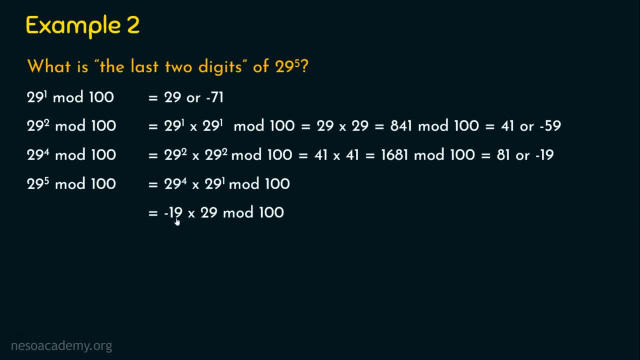 this step. So I am preferring smaller number. So I am taking minus 19 here and 29 power 1 is obviously 29.. So I am using this. When I do the calculation, I get minus 551.. When I simplify this, 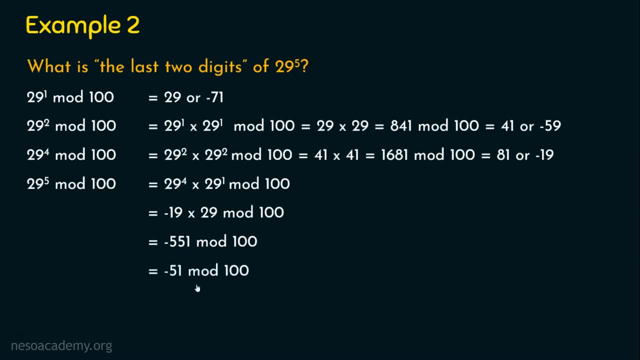 I will be getting minus 51 as the result. I already told you let the final result be represented in a positive number, right? So minus 51 plus 100.. So just add these two, we get 49 as the result. 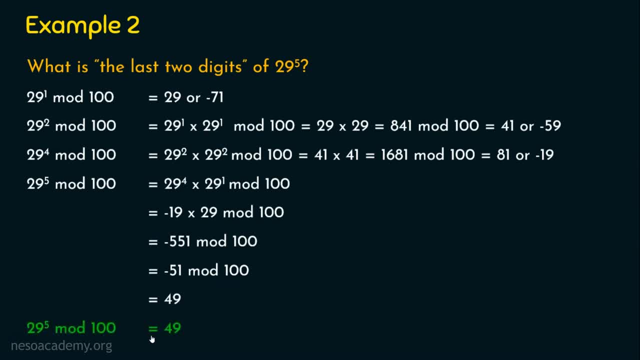 So 29 power 5 mod 100 is equal to 49.. Now you may be asking one doubt that: do we actually require this step? Instead of finding this step, we can write 29 power 5 as 29 power 2, again 29 power 2 and 29 power 1, right, I mean? 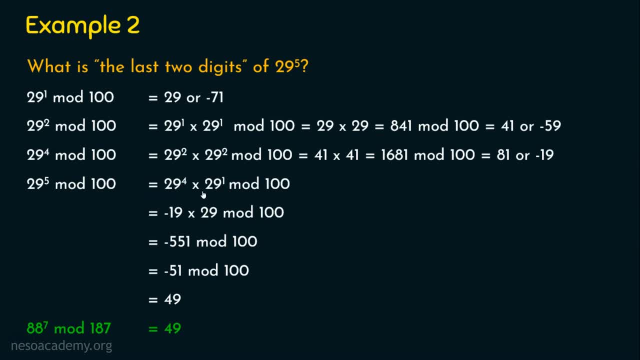 29 power 5 can be written as 29 square multiplied by 29 square multiplied by 29 power 1.. This will also give the same result, right? Of course you can do that, and that's why I told you the basic. 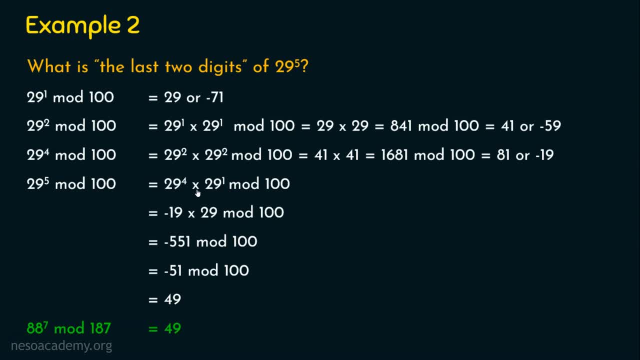 mathematical fundamental should be followed. It's up to you to decide how you are dealing this problem. In order to solve this problem, you need to know the basic mathematical fundamental. So to become proficient with these problems, I request you to try solving your own values. 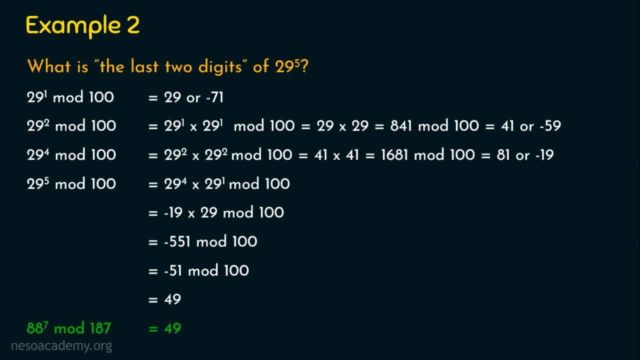 and verify it. Also, I request you to try alternative ways of solving these kind of modular exponentiation problems Like in this example. I have taken 29 power 4 as one of the steps. right, Why don't you give a try of solving 29 power 5 is equal to 29 power 2 into 29 power. 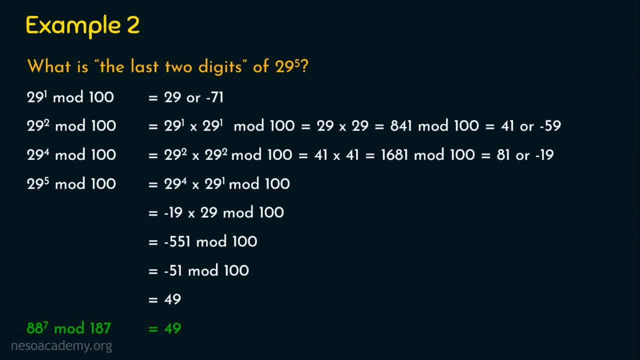 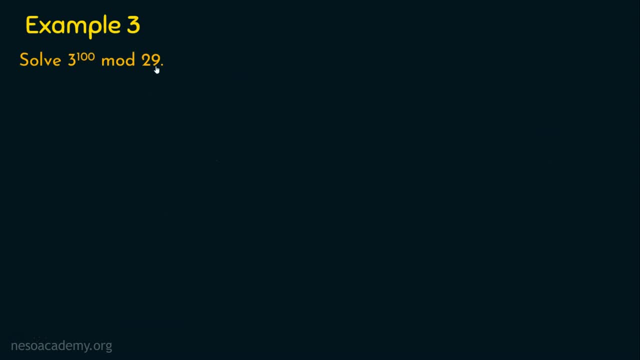 2 into 29 power 1.. Please give a try, guys. And that's it about example number 2.. Let's move on to example number 3, which is solve 3 power 100 mod 29.. So let's follow the same strategy. So. 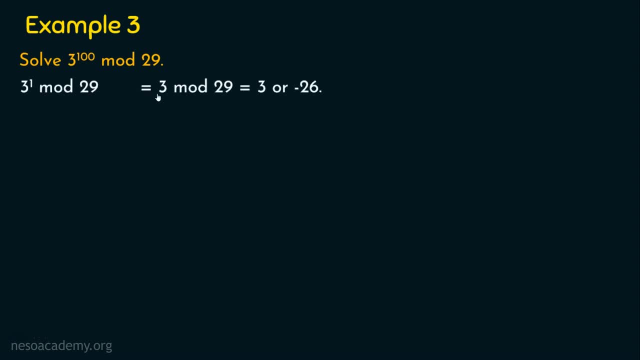 starting with 3 power 1, right. So 3 power 1 mod 29, which is equal to 3 mod 29.. So 3 mod 29 can be 3 or minus 26.. So I am just taking the positive number only. See, guys, if you are getting confused. 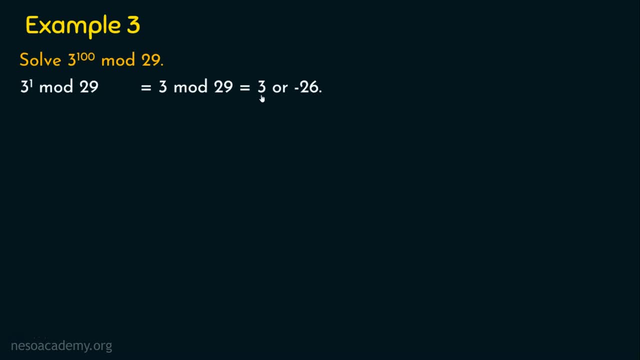 with minus values, you can just ignore those minus values and you can go ahead only with positive numbers. Ultimately, the result will be the same whether you proceed with the positive number or a negative number. So 3 power 1 we did right, So let's move on to 3 power 2.. 3 power 2 mod 29 is 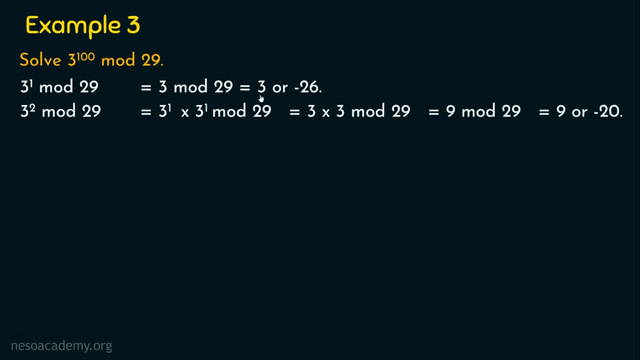 equal to 3 power. 1 into 3 power 1.. We know 3 power 1.. Which value we will take? 3 or minus 26?? Definitely 3, right? So we will take 3 into 3, which is equal to 9.. So 9 mod 29 is simply 9. 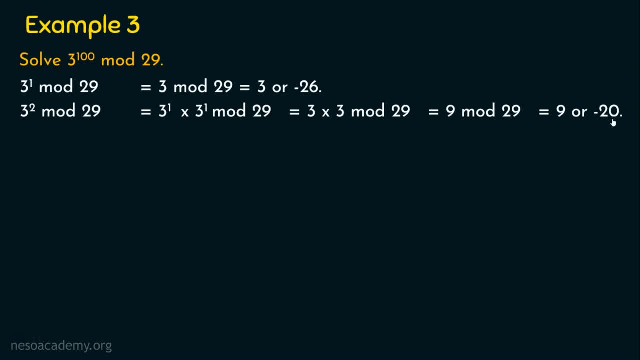 or minus 20, right. The difference between 9 and 29 is what? 20.. Since it is a smaller value, I am taking minus 20 here. Anyway, 9 is going to be preferred. This step is actually 3. 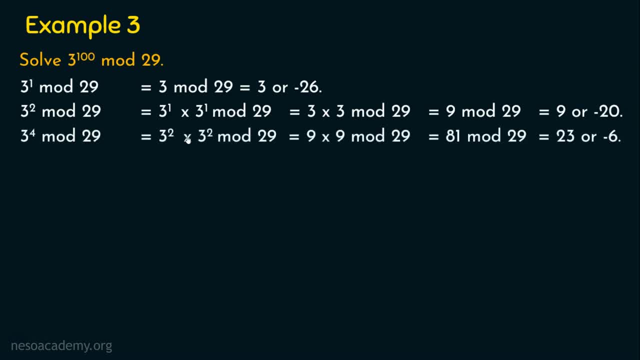 power 2.. The next step is going to be 3 power 4.. 3 power 4 can be written as 3 power 2 into 3 power 2.. We know 3 power 2 is what 9.. So 9 into 9, which is equal to 81 mod 29.. So 81 mod 29 is. 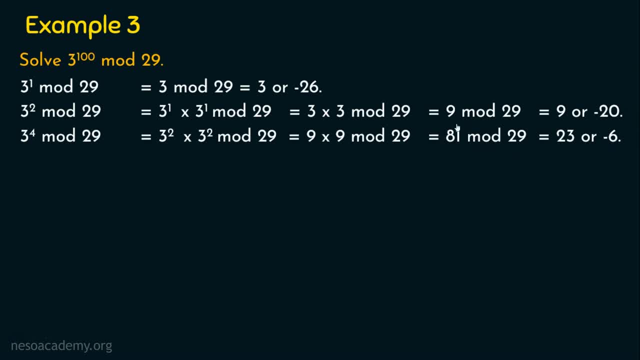 equal to 23 or minus 6.. So when you divide 81 by 29,, the remainder will be 23.. Do we need 23?? So it means 23 mod 29.. Are we going to take 23 or we can reduce it? We can represent this as minus. 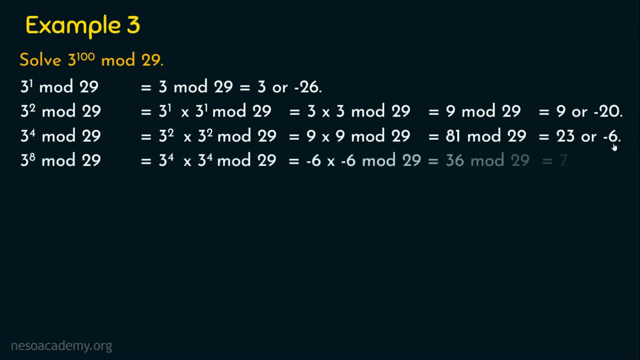 6.. So let this be minus 6.. The next step is equal to 3 power 8.. 3 power 8 is 3 power 4 into 3 power 4.. So in the previous step, 3 power 4 is what? Either 23 or minus 6.. Since this is a smaller number, I am taking minus. 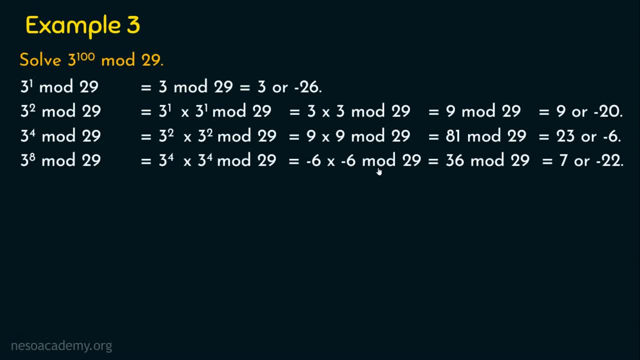 6. So the simplification will give me minus 6 into minus 6, mod 29, which is equal to 36, mod 29, which is equal to 7 or minus 22.. I am not going to focus on minus 22, because 7 will be easy for. 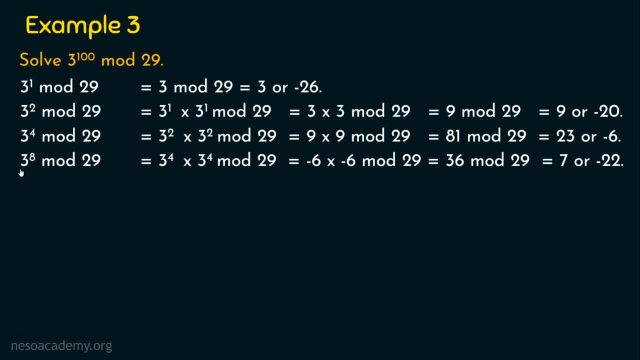 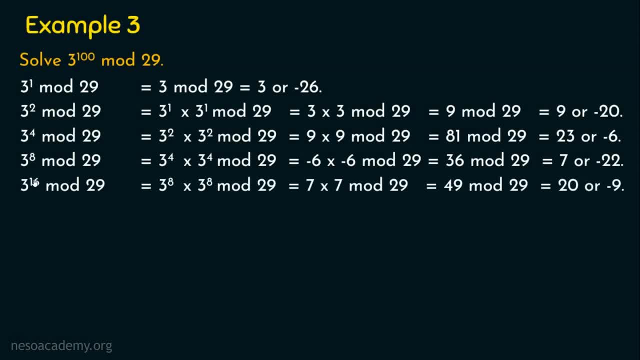 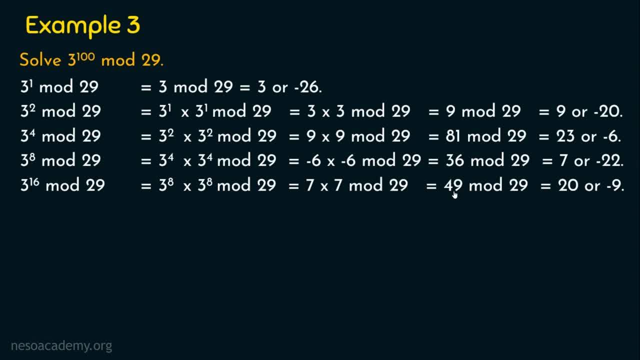 step. we calculated 7.. So 7 into 7 mod 29, which is equal to 49 mod 29, which is 20 or minus 9.. Right, We are now in 3 power 16.. Let's do 3 power 32.. 3 power 32 is 3 power 16 into 3 power 16, which. 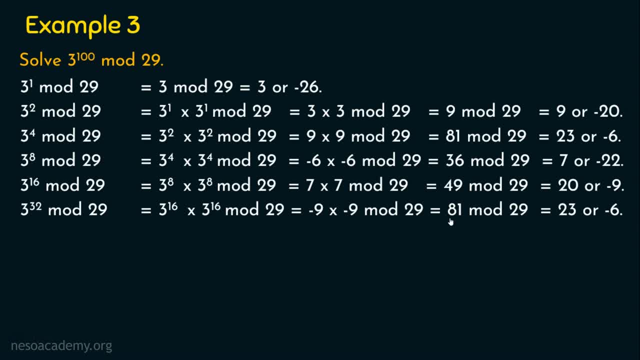 is equal to minus 9 into minus 9.. This value I am taking, which is equal to 81 mod 29, which is 23 or minus 6.. Can you see here? Then we are going to do 3 power 64. So 3 power 64 mod 29 is equal to. 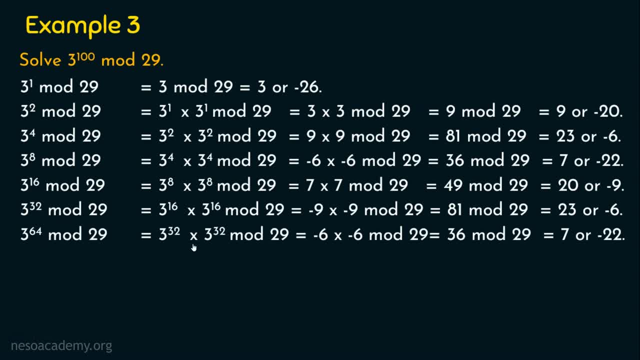 the previous step, Right 3 power 32.. So 3 power 32 multiplied by 3 power, 32 mod 29.. 3 power 32 is minus 6.. So minus 6 into minus 6 mod 29 will give 36 mod 29, which will give 7 or minus 22.. Then we 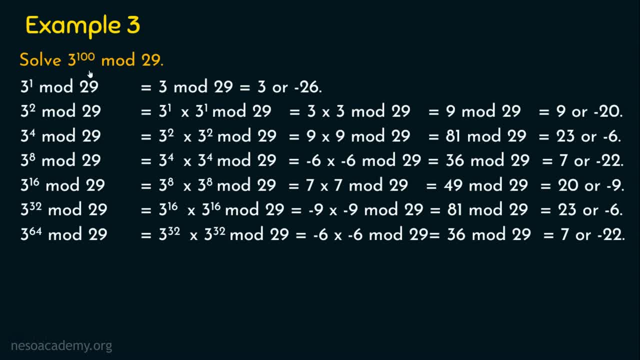 are not going to proceed with 3 power 128, because the question is actually 3 power 100.. So I am going to get 3 power 100.. So I am going to proceed with 3 power 128, because the question is actually. 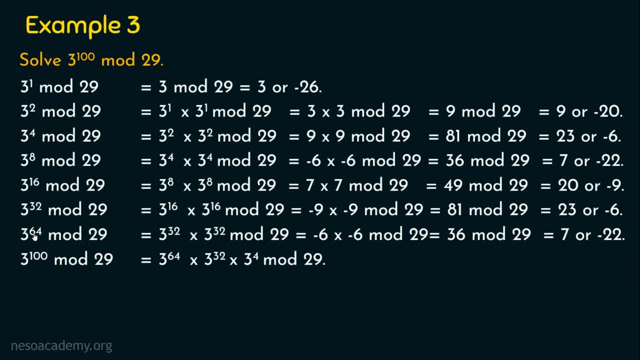 3 power 64. Then 3 power 32.. So 64 plus 32 is 96, and we need 4.. Right, So we will take this. So 3 power 100 can be written as 3 power 64, which is this, 3 power 32, which is this, and 3 power 4. 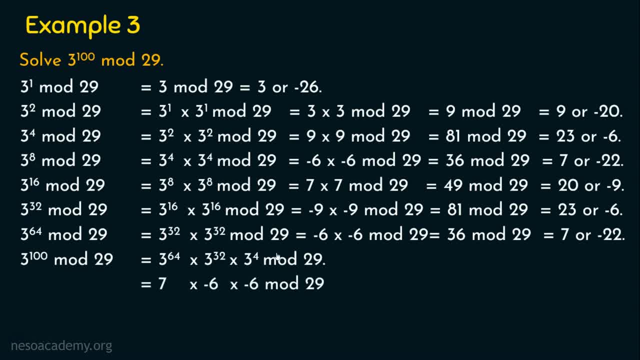 which is this. So I am just substituting the equivalent values. 3 power 64 is actually 7.. I am taking this 7.. 3 power 32 is actually minus 6.. I am taking this minus 6.. 3 power 4 is also. 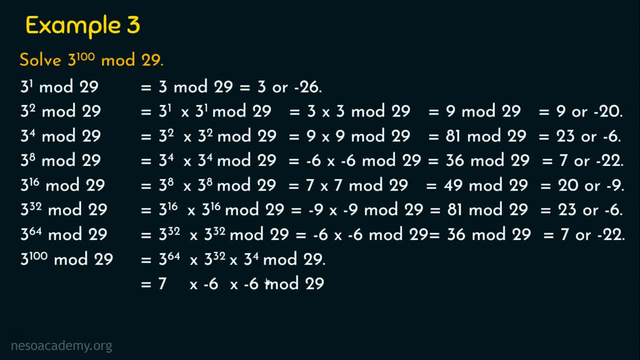 minus 6.. Right, So 3 power 4 is also minus 6.. So I am taking this minus 6.. So I am taking this minus 6.. So 7 into minus 6, into minus 6, will give a positive number, because we have 2 minus here. 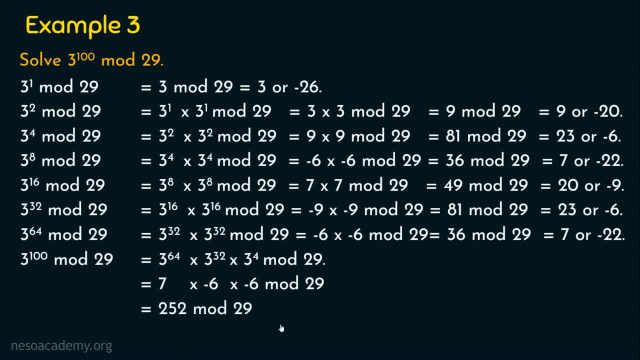 So we get 252 mod 29.. 252 when it is divided by 29,, we get the remainder 20.. So the answer for 3 power 100 mod 29 is 20.. Let's see the last question, Example number 4, which is solve 23. 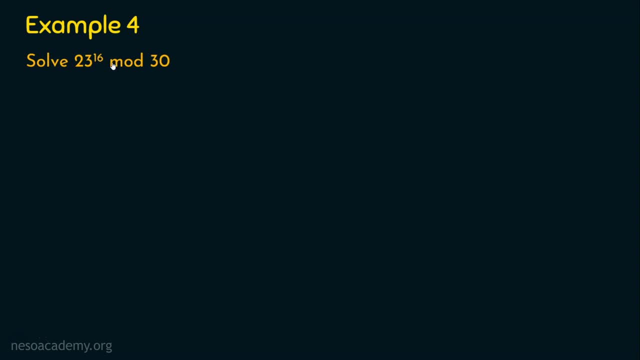 power 16 mod 30. Can you see here, this is 23 power 16 mod 30. You can also simplify this as minus 7 power 16 mod 30. So you can also simplify this as minus 7 power 16 mod 30. So you can also simplify. 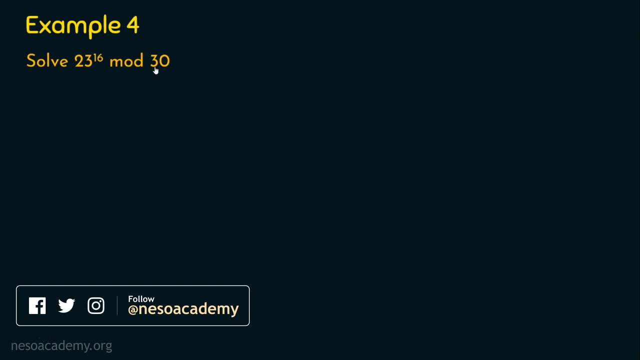 this as minus 7 power 16 mod 30. So you can also simplify this as minus 7 power 16 mod 30, because we can write 23 mod 30 as either 23 or minus 7.. So you can solve this in any way, but the intention of 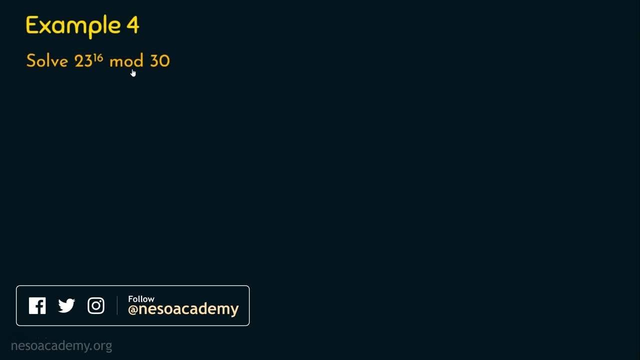 this example is to show there are many ways to solve this problem Right? Just see here how I am solving. So 23 power 16, mod 30 is written as 23 power 2, the whole power 2, the whole power 2. 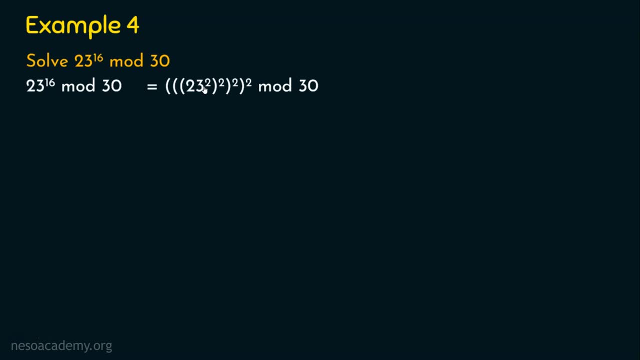 and the whole power 2.. So 23. we have powers here, Right? Just multiply these powers 2 into 2 into 2 into 2. So this is 16.. So actually, this is 23 power 16 mod 30. So this is 23 power 16 mod 30. So this is 23 power 16 mod 30. So this is 23 power 16 over here, and this is 23.. So we have그래pto 3 fought 16.. So this is 23 power 16.. I am writing 23 per 16, which is thisO 23 power 13.. I am writing. 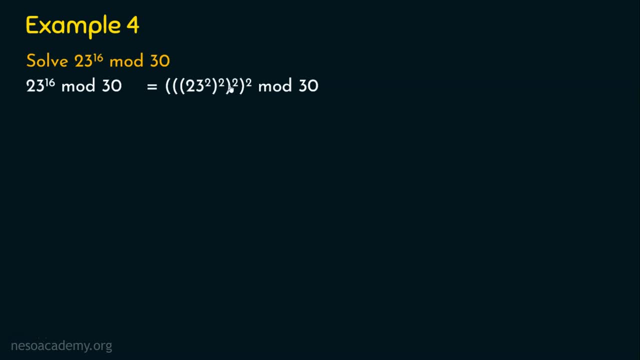 23: 0, which is thisせて: 2, 3 square, the whole square, the whole square, the whole square. mod number 3 per square: the whole square, the whole square, the whole square. お30 remainsthe same. 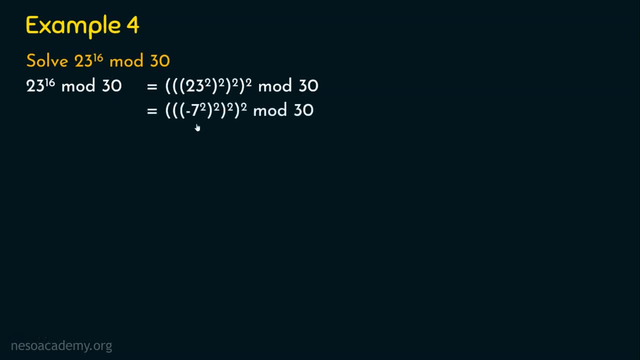 Now we can reduce this Right: 23 and 30. We can reduce it as minus seven. So 23 is 23snd 30. So 23 is rerisen as minus seven. This 2 remains the same and we have all 4 2s on. 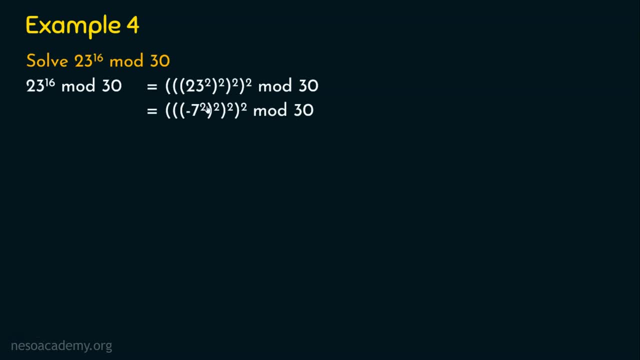 the powers. So we have this now. Then we can easily simplify: is now: what is this value him for 12,? what is this value minus 7−0-7 square can be written as 49.. Right, So am 49,. right, So I am just replacing this with 49.. Still, we have three 2s on the power, correct? 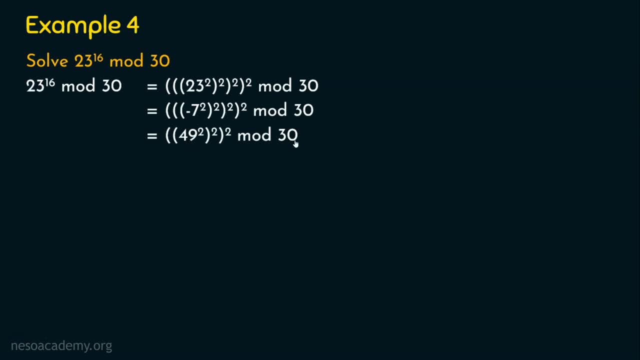 So 1,, 2,, 3.. Now we will reduce this 49 and 30. We can reduce it as 19,. right 49, when it is divided by 30, we get the remainder 19.. So I am just replacing 49 with 19.. We have these three 2s. 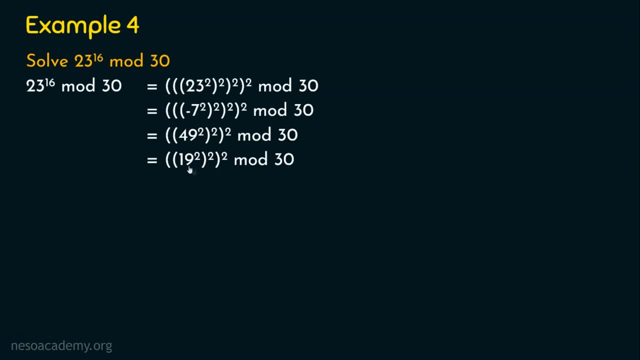 on the power again. So 19 or 30.. We can either do 19 square or we can still reduce it, right? So 19 mod 30 can be either 19 or minus 11, right, Since minus 11 is smaller, I am taking minus 11.. 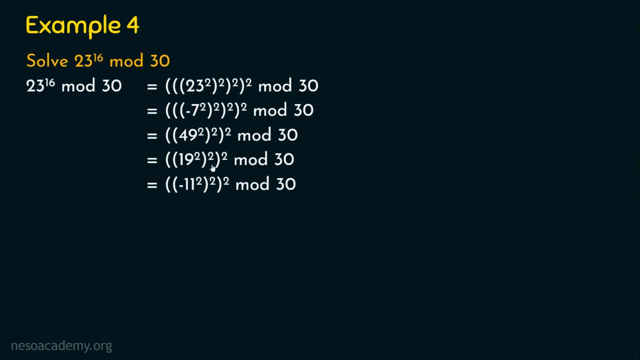 So 19 is simply replaced as minus 11.. We have three 2s on the power, just like that. Now we can reduce this Minus 11 square is 121, right, So 121.. So this 2, this power 2 is reduced to. 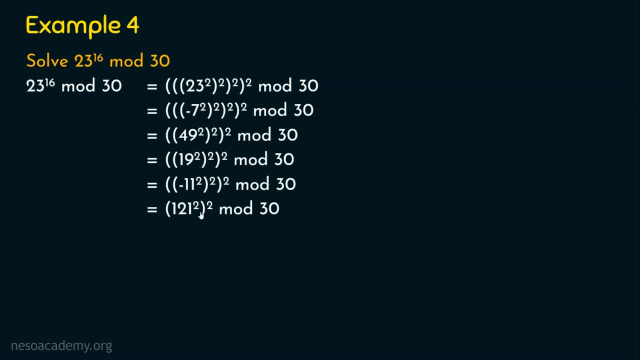 this. We still have two 2s right On the power, these two 2s. Now we will reduce this 121 mod 30. We get 121.. When it is divided by 30, we get the remainder 1.. 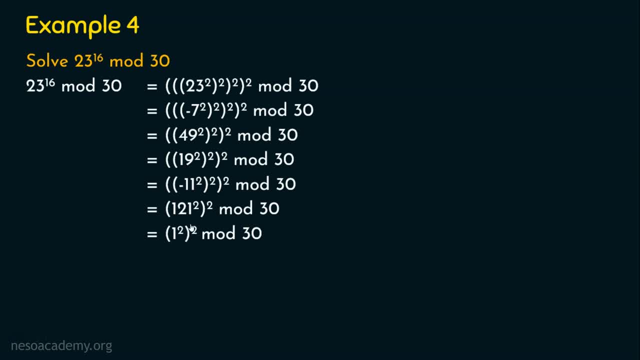 We have two 2s on the power right. Still we are having two 2s, So 1 power. any number of 2s will give remainder 1, and 1 mod 30 is definitely 1.. So the answer for 23 power, 16 mod 30 is simply: 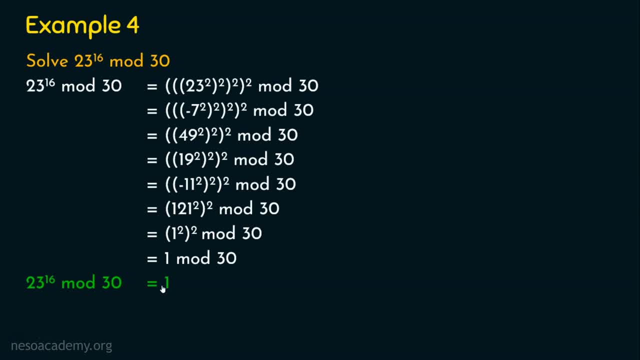 1.. The intention of showing example number 4 is: we have so many ways to solve a problem. You can choose any approach in which you are comfortable with. Before we sign out, let's see the homework questions. There are two questions. The questions are solve. 11 power 23. 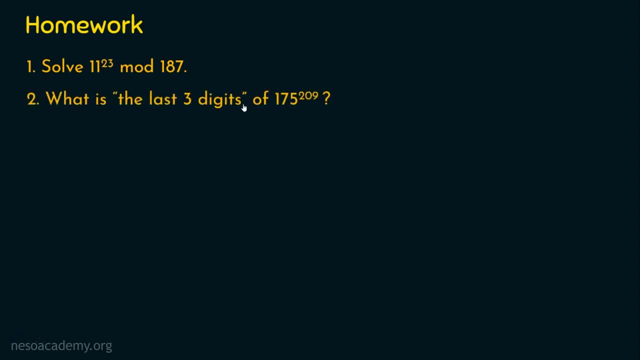 and the second question is: what is the last three digits of 175 power 209?? So we are going to find last three digits, right. So it means we are going to solve 175 power 209 mod 1000.. I request. 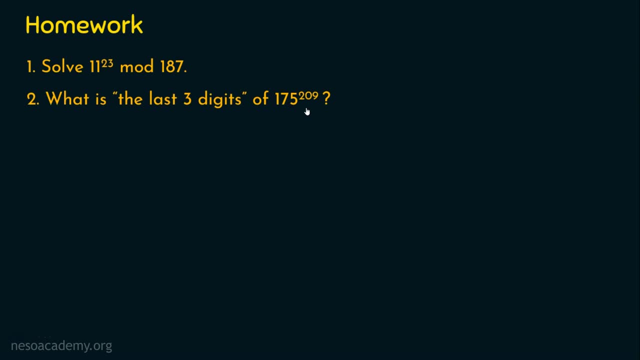 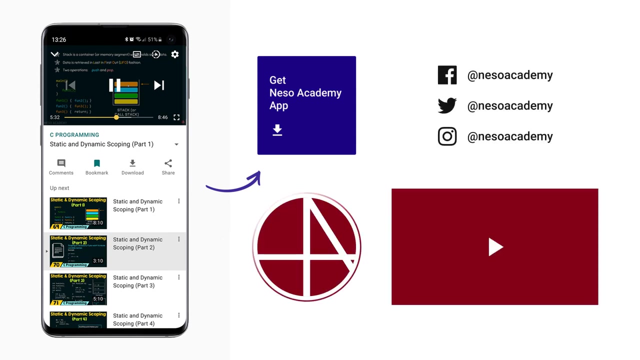 you to solve these problems and post your answers in the comment section. And that's it, guys. I hope now you understood modular exponentiation with examples. Until I see you in the next presentation, thank you for watching. Thank you for watching.